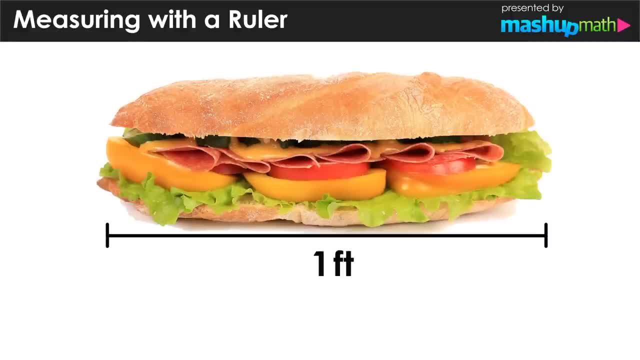 foot long. Now you probably already know that one foot is exactly the same thing as 12 inches. They are two different units of measurement and if we cut this sandwich directly down the middle in half, we know that each half would be six inches long. And for this lesson we are going to explore using 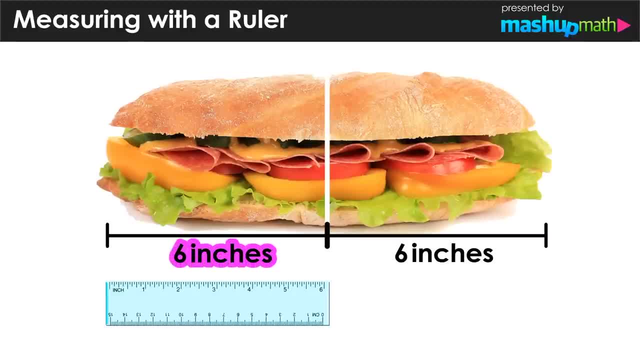 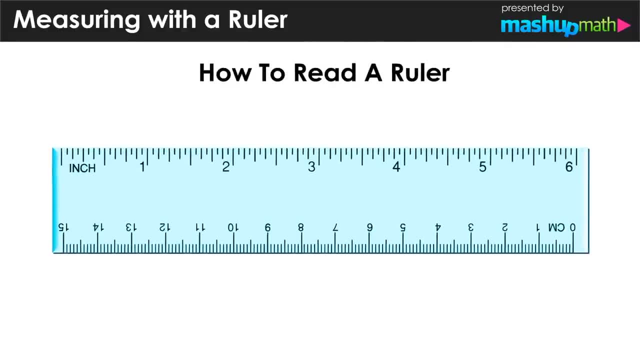 a ruler that has that same length of six inches and we're going to take a look at what the symbols and markings on the ruler mean And how we can use them to measure different sized objects. So let's take a look at the side of the 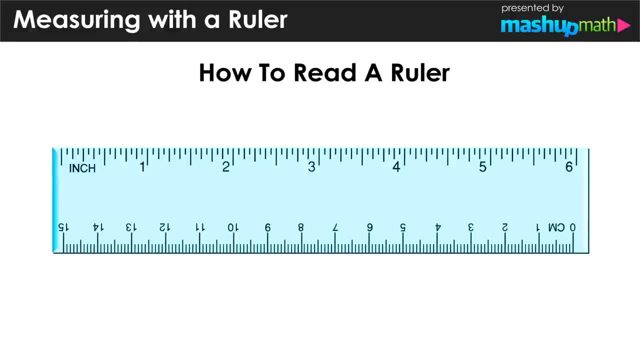 ruler that's labeled in inches and you can determine that by looking for the word inch or IN as an abbreviation. Notice the large numbers one through six are labeled on the ruler. Each of these spots is a value of one inch in length, So the distance between zero and one is equal to. 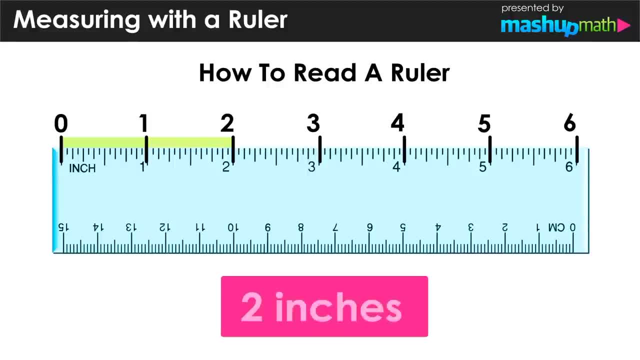 one inch inch. The distance between 0 and 2 is equal to 2 inches, which can be expressed as 2in. The distance between 0 and 4 would be equal to 4 inches. But what would happen if we're? 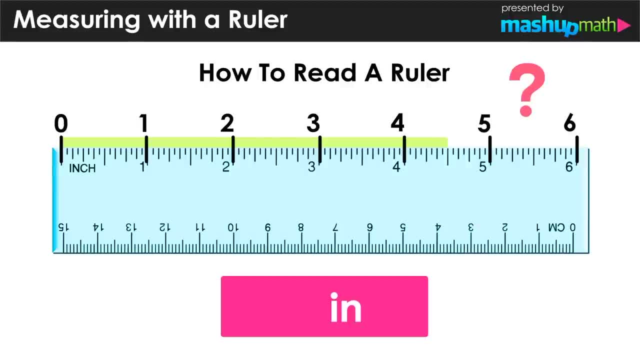 measuring a distance that falls somewhere in between two of these values. Notice that there is a marking directly in between each 1 inch marker on the ruler, and each of those markings are going to represent 1 half, so in this case we have a length of 4 and 1 half. 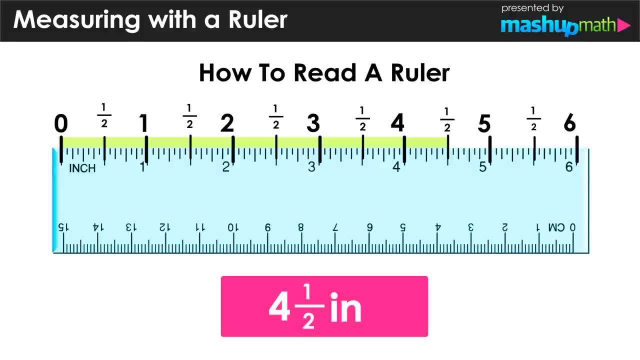 inches. Now what if we push our measurement a little bit further, so that it's in between a whole number and a 1 half? In this case we're in between 5 and 5 and a half. The markings in between these values are each worth 1 quarter. so in this case we 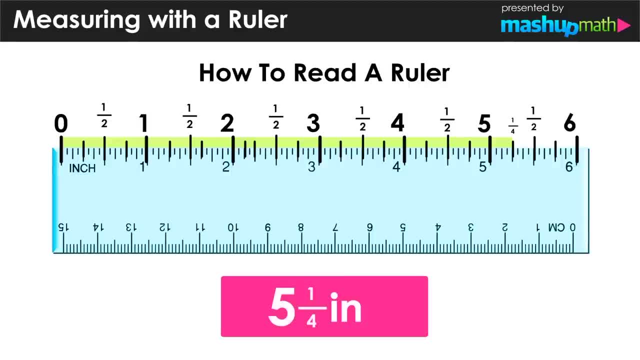 have a measurement of 5 and 1 quarter inches, or 5 and 1 fourth, And if we push our length a little bit further, so that it's in between one half and the next whole number, we can conclude that this length is equal to 5 and 3 quarters or 5 and 3 fourths. 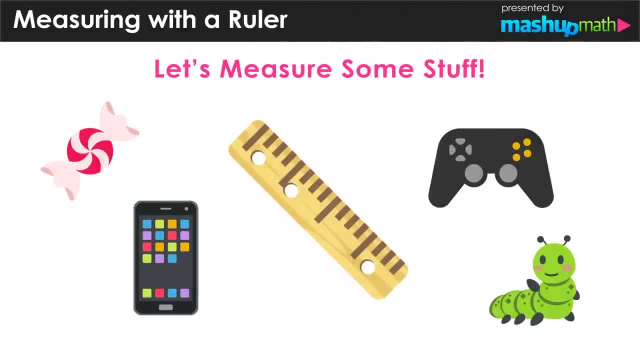 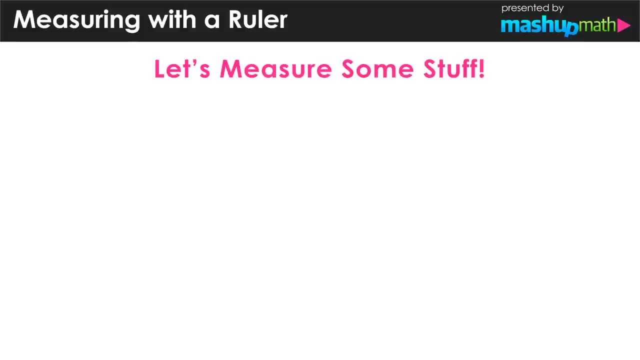 So, now that you have a better understanding of using a ruler to find the measure of a length, let's gain some practice using a ruler to measure some different items. So let's start off by finding the height of this piece of candy. We can start by turning. 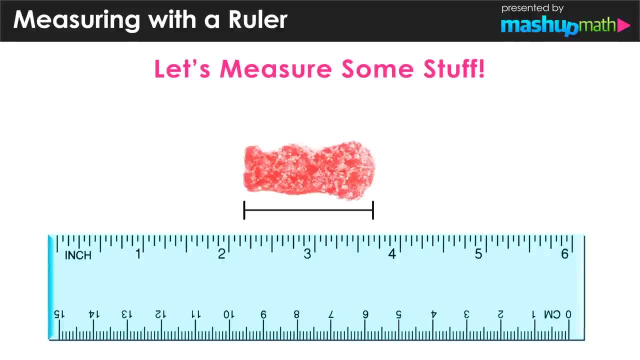 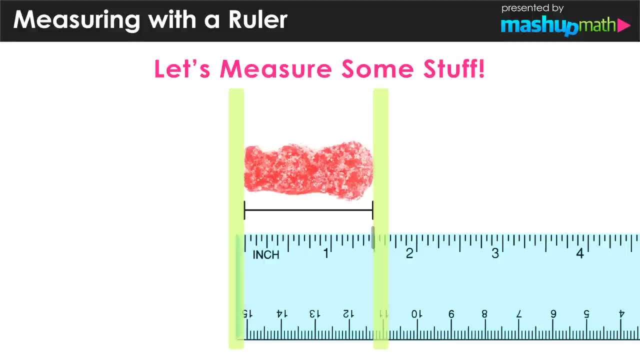 the figure on its side and taking our ruler and lining it up so that the 0 inch mark is aligned with the left edge of the figure and seeing how far along it goes on the ruler to the right edge of the figure. In this case, this piece of candy has a length of 1 and a half inches. 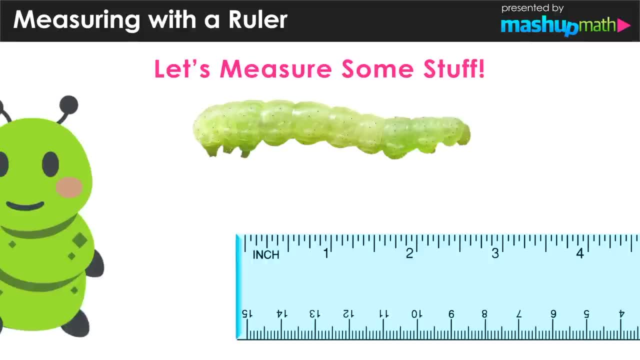 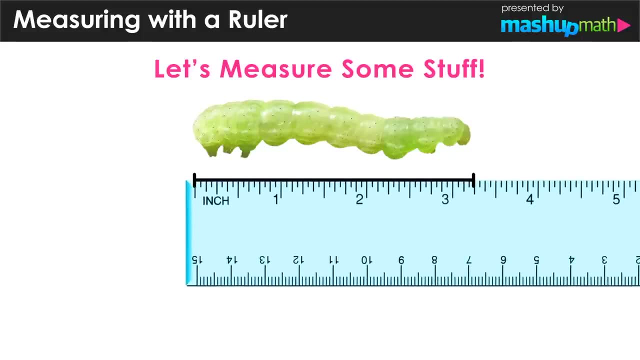 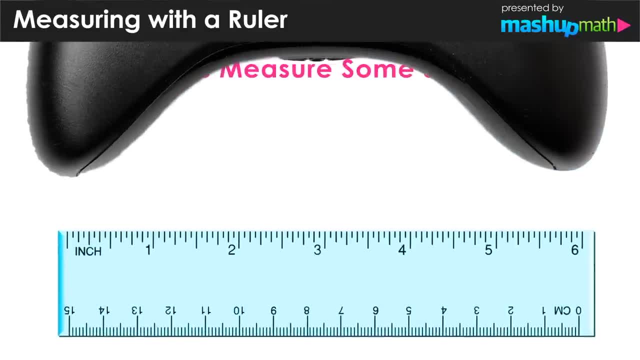 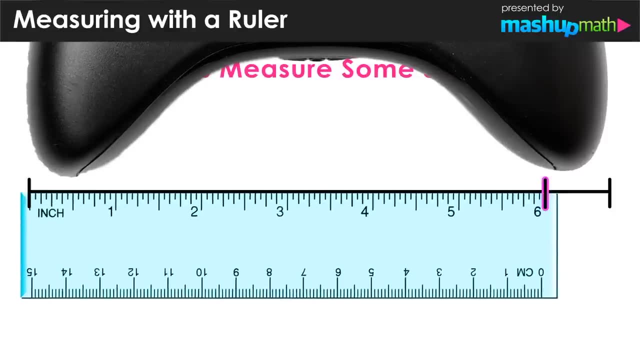 Again, we want to use our ruler to find the length of this object. so we can line our ruler up on the left edge at the 0 inch mark and we can see that this object is longer than 6 inches. So first we measure the first 6 inches of the object and then we have to measure the 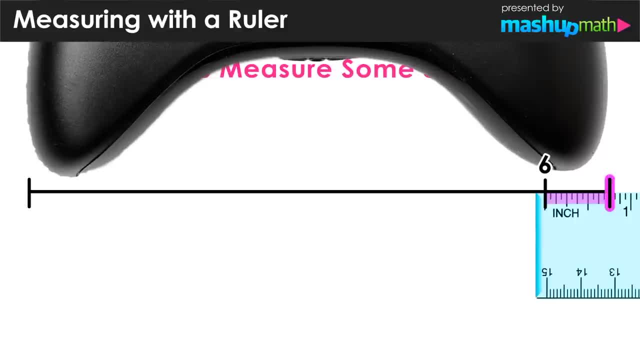 length of the extra space. To do that, we can slide our ruler over and see that this figure extends an extra 3 quarters of an inch. so we can conclude that the video game controller has a length that measures six and three quarters of an inch. so this should get you comfortable now with using your ruler to find the length of. 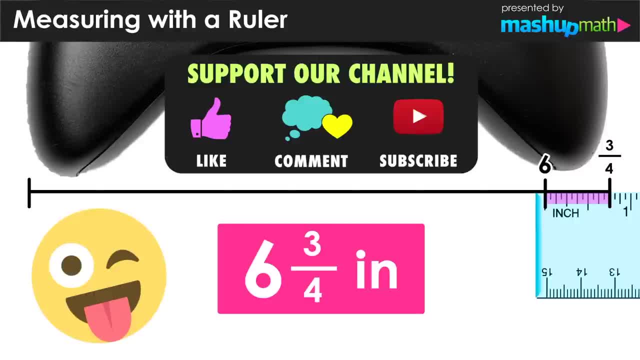 measurements of different objects. so you might want to go back and re-watch this lesson a few more times and continue practicing using your ruler as you continue to explore measurement and different topics in mathematics, and I thank you again so much for stopping by. I hope you had fun. 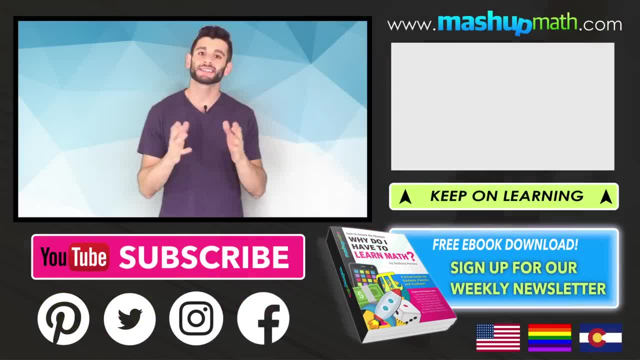 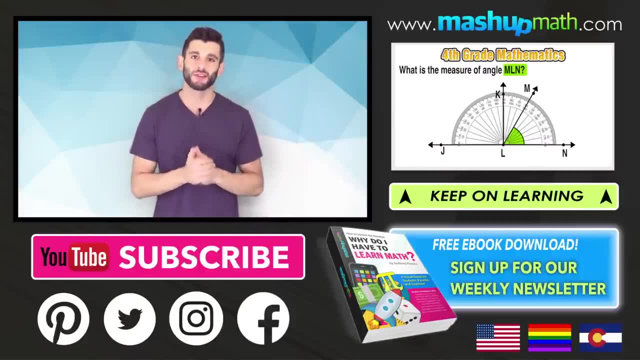 and I'll see you all next time. all right, so that's it for this lesson. thank you again for stopping by. I hope you found it helpful and, if you did, please click that link below and subscribe to our YouTube channel. leave a thumbs up and a comment on this video. we could really use your. 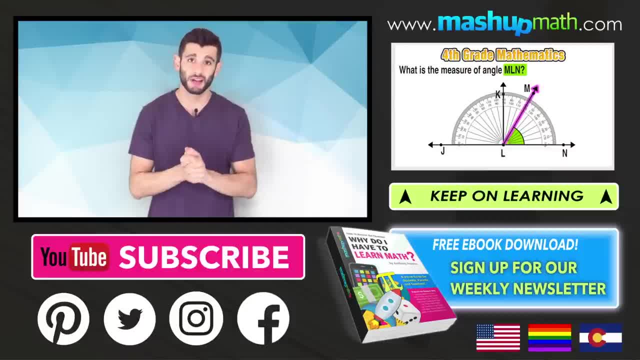 support. and also don't forget to sign up for our weekly newsletter. when you join our mailing list, you get a free ebook download, as well as weekly resources, tips, insights and some cool contests and giveaways as well. Thanks for watching, so don't miss out on that. there's a link on this page you can click to join the mailing list and 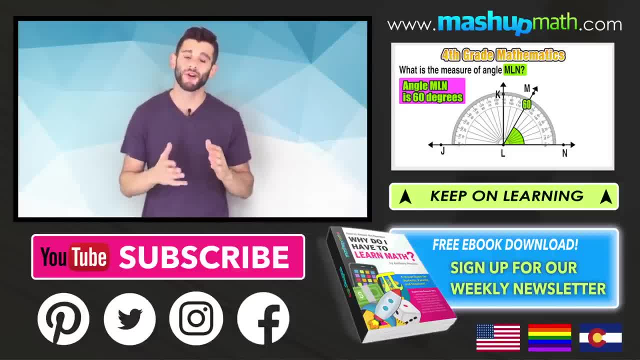 that's all you have to do, so thank you so much again for stopping by and for all your support, and I will see you all next time. bye. 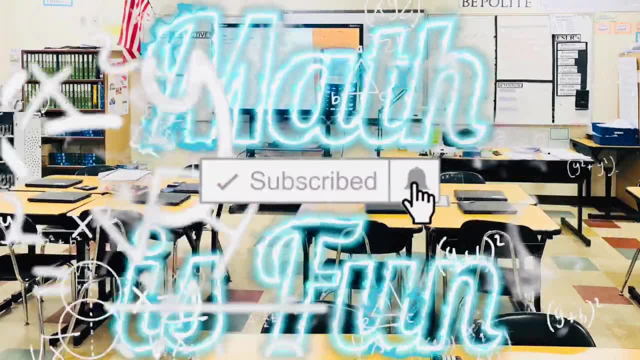 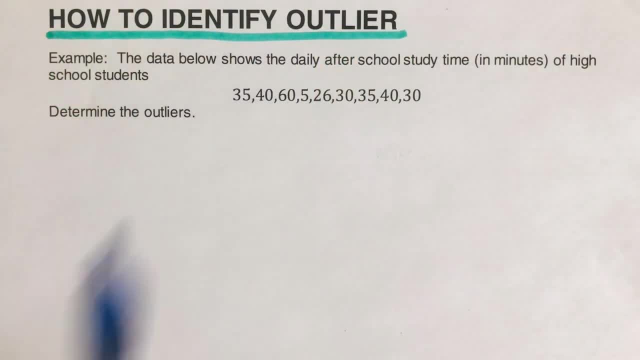 Hello everyone, In this video we are going to identify outliers. What is an outlier? Outlier as a word comes from two words combined together: It comes from the word out and lie. So this means that these are the values that lie outside most of the other values in a data set, which means: 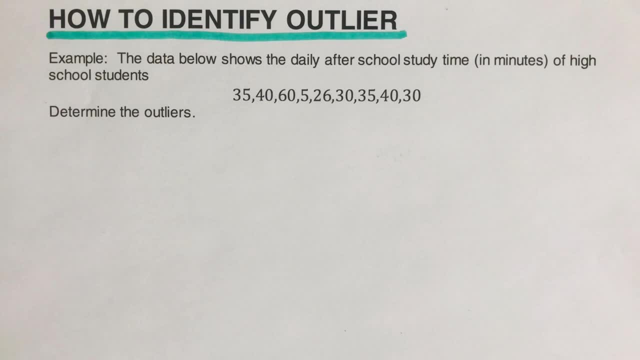 that if we say outlier, these are values that are way too small or way too big or too large compared to the rest of the value. Now let's take this example right here. There are some steps that we need to follow in order that we can objectively determine an outlier from a set of data. So we 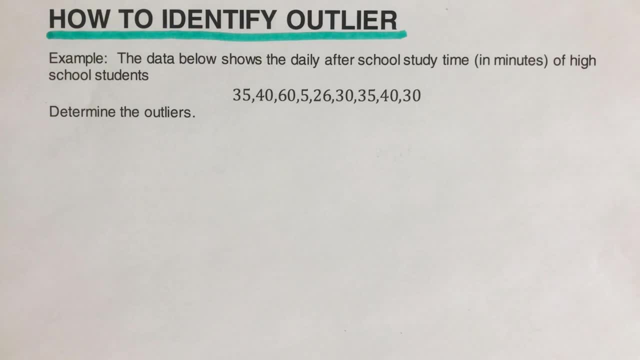 don't just say, oh, this is way too big, I can take this as outlier, or this is way too small, I'll just take this as an outlier. So there are steps that we need to do so that we can objectively determine which ones are outliers and which ones are outliers. So let's take this example right here.